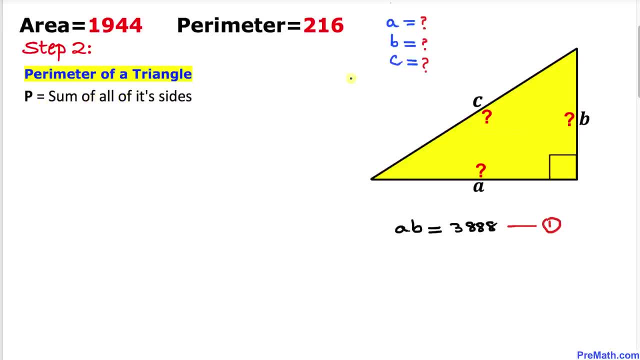 equal to the sum of all of its side lengths, and our side lengths are a, B, C and our given perimeter is 216, so I can write this one as a plus B plus C, equal to 216. Now let me go ahead and call this as an equation number two. 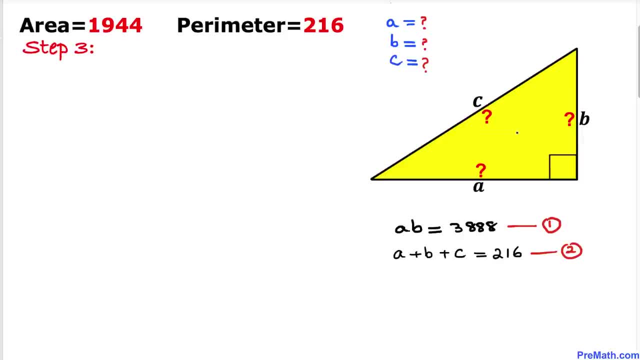 And here's our next step, since we are dealing with this right triangle. Oh, therefore, let's recall the Pythagorean theorem: a square plus B square equal to C square. Let me go ahead and write down: a square plus B Square equal to C square. now let me go ahead and call this as an equation. 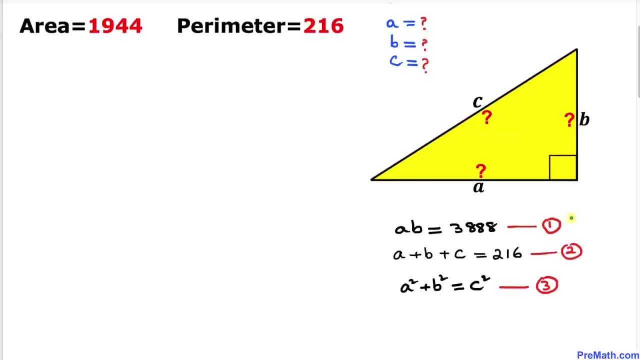 number three. and now we got these three equations, as you can see, and now we are going to solve for A, B and C. and here's our next step. Let's recall this well-known formula: a plus B square equal to A square plus B square plus 2 Ab. 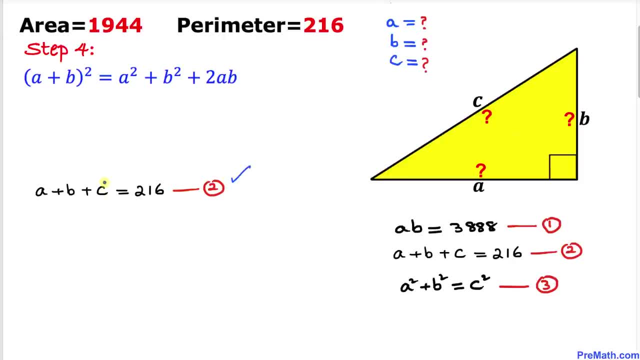 No, let's recall this equation number two: if I move this C on the other side, this A plus B equal to 216 minus C. but therefore this A plus B I am going to replace by 216 minus C and this A square plus B square I am going to replace it. 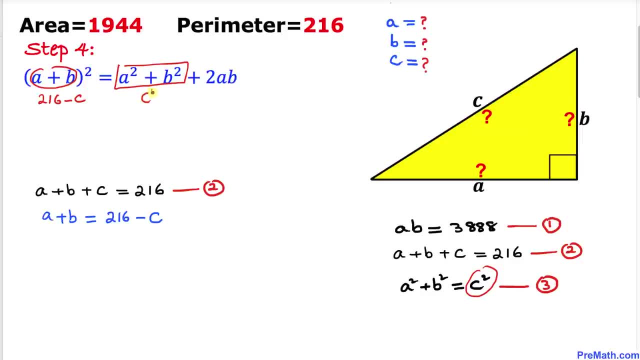 by C square. so I'm going to replace it by C square, and here, a times B, I am going to replace it by three thousand eight hundred and eighty eight, so therefore I can write this one, two, so I am going to make it 517 minus 2. 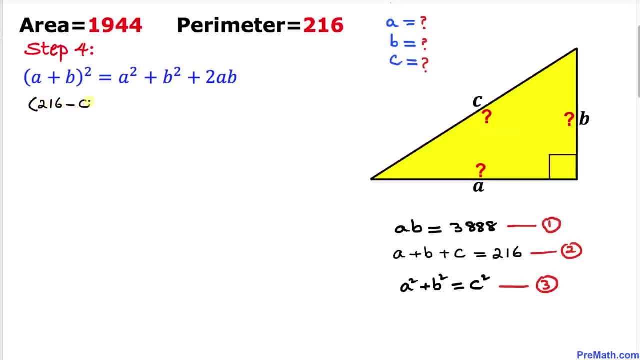 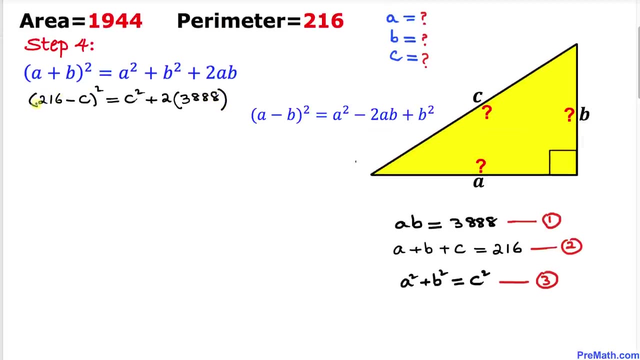 so, therefore, I can write this: one two 216 minus C, whole square equal to C square plus 2 times 3888. and now let's go ahead and expand this binomial on this left-hand side by using this formula, so this could be written as 216 square minus 2 times 216 times C, and. 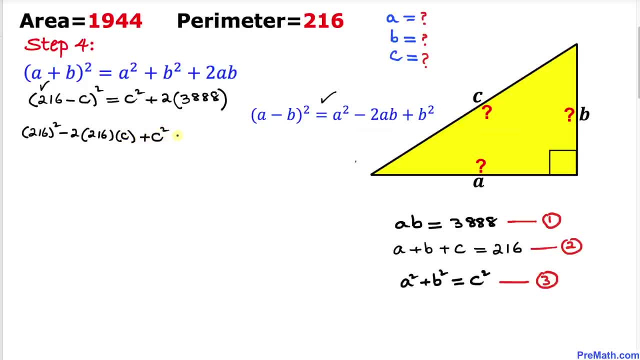 then plus C square- and on the right-hand side I can write C square- plus 2 times 3888 is going to become 7776. and here's our next step. once we took care of this square of 216 and multiplied these one out, now we can see this C square on this side and this C. 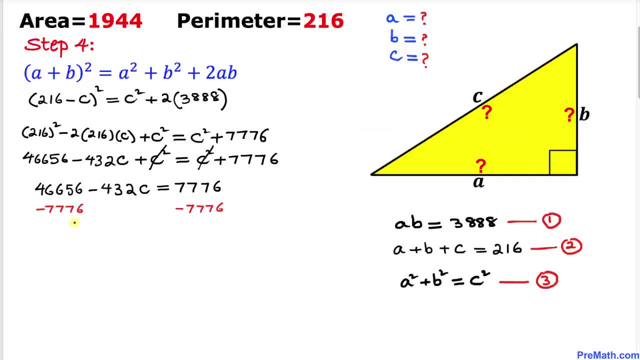 square, they cross each other out. and now let's go ahead and subtract seven thousand seven hundred seventy six from both side. they are gone. so we ended up with the three. seven, seven, six. and now let's go ahead and subtract seven thousand seven hundred seventy six from both side. they are gone, so we ended up with three. 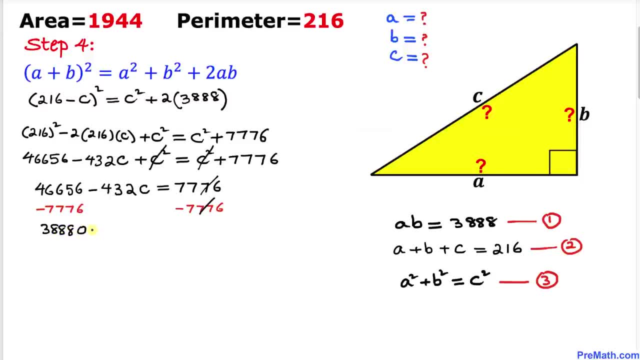 eight eight eight zero minus four hundred and thirty two C equal to zero. and now let's go ahead and move this 432 C on the other side. and now let's go ahead and divide both side by 432 on this side and 432 on this side to. 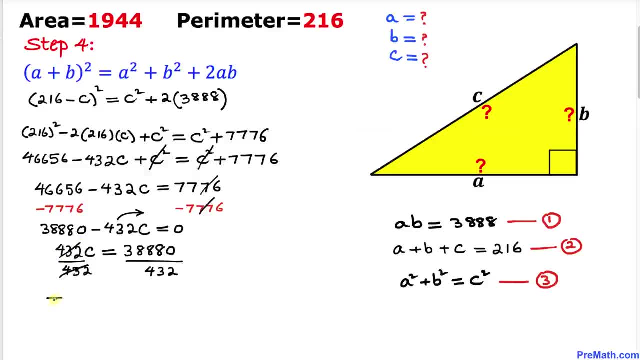 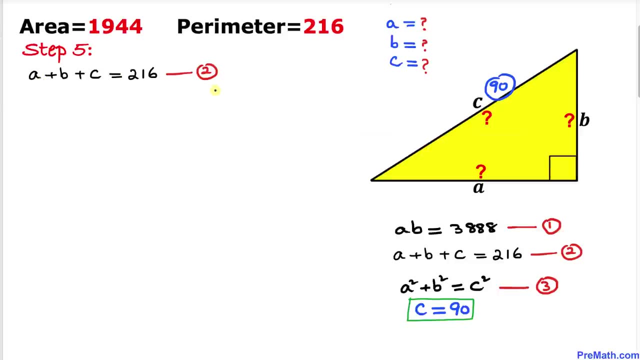 isolate C, so this is gone. so our C value: if we divide this one turns out to be 90, so our side, C turns out to be 90. and here's our next step. let's recall this equation to a plus B plus C, equal to 216, and we know that our 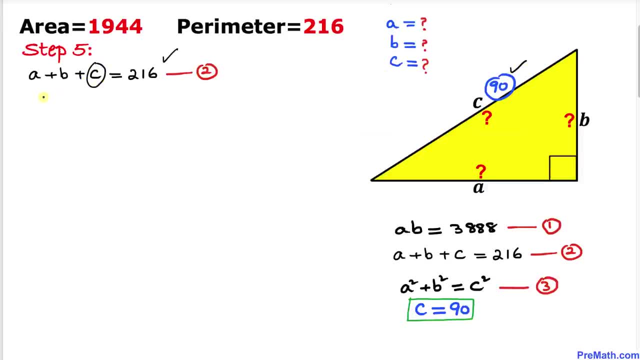 C value turns out to be 90, so I can write a plus B plus 90 equal to 216. now let's go ahead and subtract 90 from both side. this is gone. so our a plus B value turns out to be one hundred and twenty six. let me go. 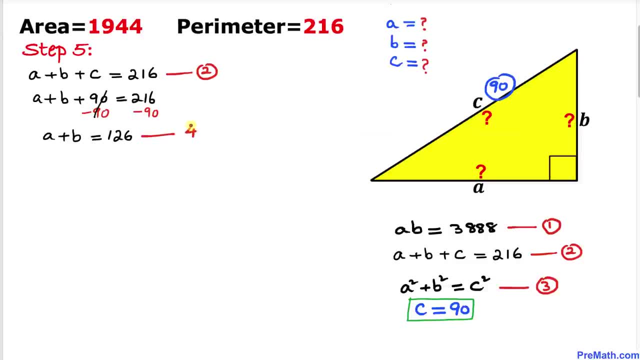 ahead and call this equation as equation number four. and now let's focus on this equation, one which I just wrote down: a times B equal to three thousand eight hundred and eighty-eight. let me go ahead and divide both side by a, divide by this side, a as well. so a and a is gone, so our B value turns out to be three eight. 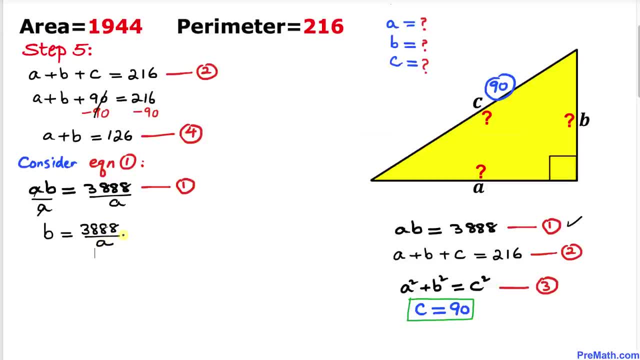 eight, eight divided by a. and now let's plug it in this: B equal to value three, eight, eight divided by a, in this equation, four. so let's go ahead and fill in the blanks. so a plus B. I'm going to replace it by this: one, three, eight. 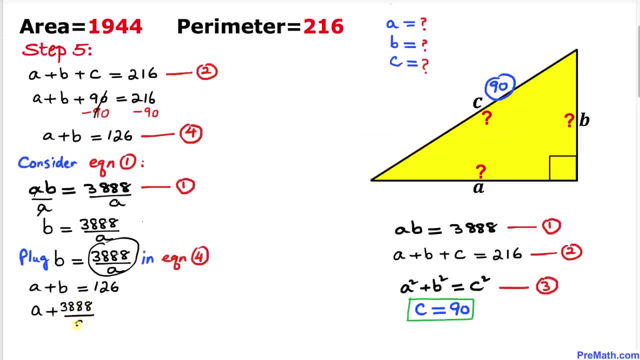 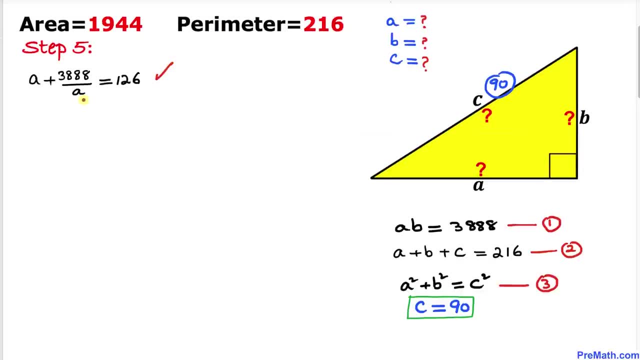 eight. eight divided by a, equal to one hundred and twenty six. and here's our equation. let's go ahead and solve for a. first of all, we want to remove this fraction, so let's go ahead and multiply by a across the board. so this a times a. 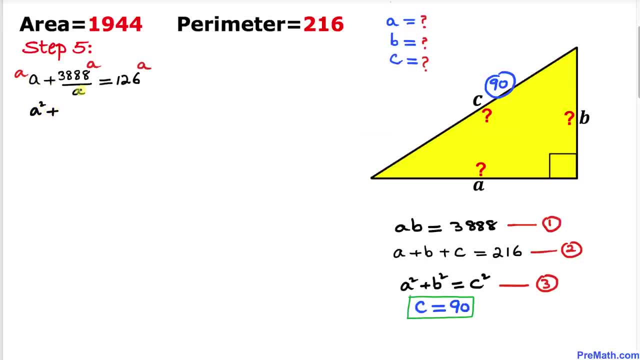 is going to become a square plus this a and a is gone, so we got 3888, equal to 126a. and now let's move this 126a on the left hand side. so we got this quadratic equation: a square minus 126a plus. 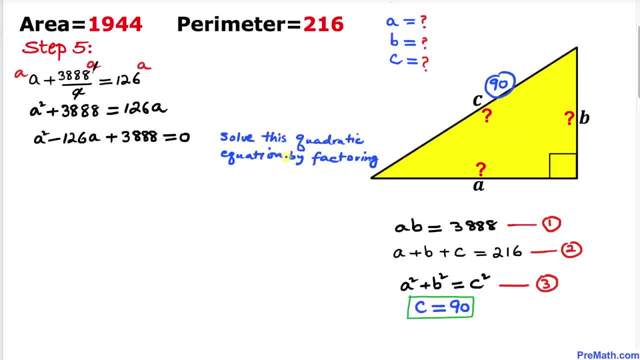 3888 equal to zero, and now we are going to solve it by factoring. in order to find the factors, let's focus on this constant, part, 3888. i have just copied it down. now we know that this number is divisible by eight. according to this divisibility by eight rule, a number is divisible. 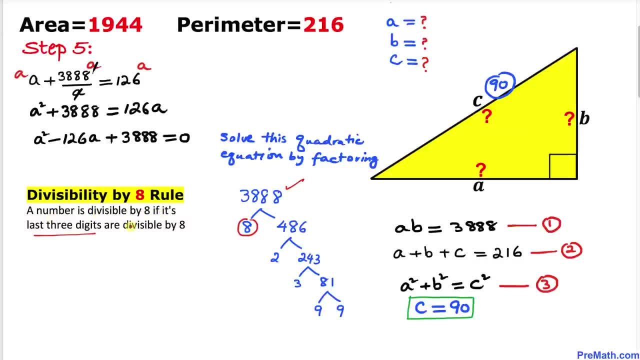 by eight, if its last three digits are divisible by eight, and the rest of these factors are pretty simple. so we found out the factors of 3888 as 8, 6, 9 and 9. now we can easily see that a times 9 is 72 and 6 times 9 is 54. 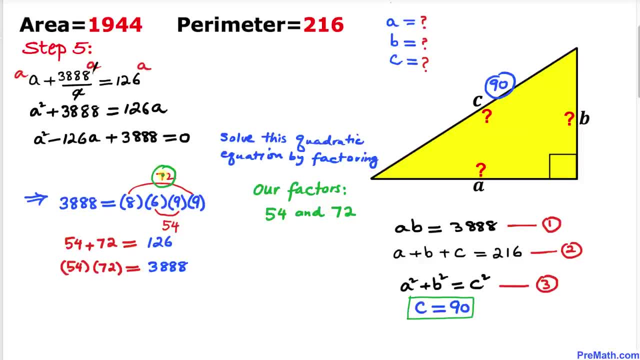 so thus our factors turn out to be a 72 and 52- 154. if we add these two numbers, we are going to get 126, which is right here, and if we multiply them, we are going to get 3888, which is this number. So thus our factors turn out to be a minus 54. 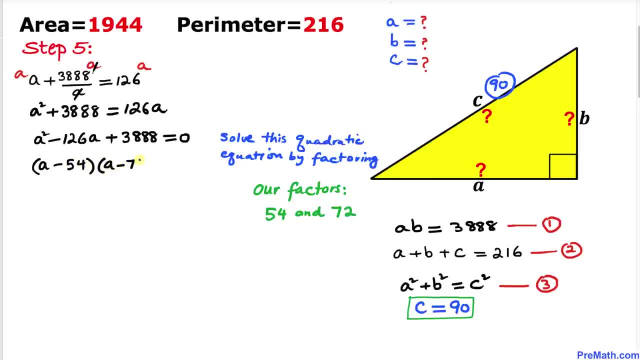 times a minus 72 equal to 0. and now let's go ahead and separate them: a minus 54 equal to 0, and this one a minus 72 equal to 0. So our a value turns out to be 54, and here our a value is. 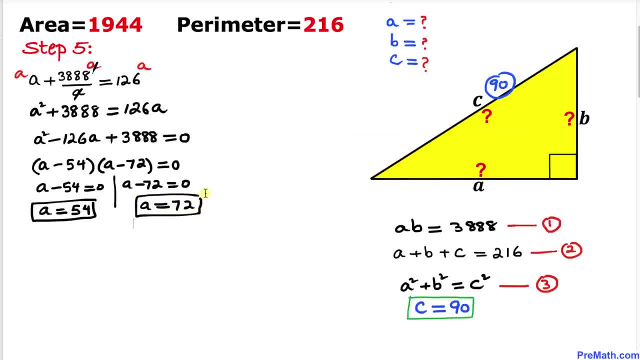 72.. And here's our final step. we got a equals to 54 on this side and we already figured out c equals to 90 and our other value of a is 72, and I put down c equals to 90 as well. and here's our equation. 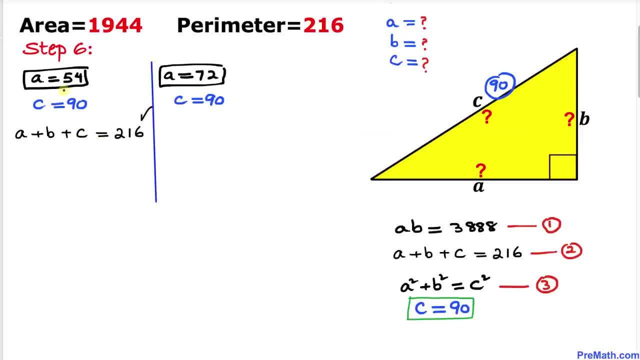 number two. Let's go ahead and fill in the blanks to find the value of b. Our a value is 54 plus b plus c, c is 90 equal 216. and finally, we figured out our b a value as 72. So in this case, our a value is 54. 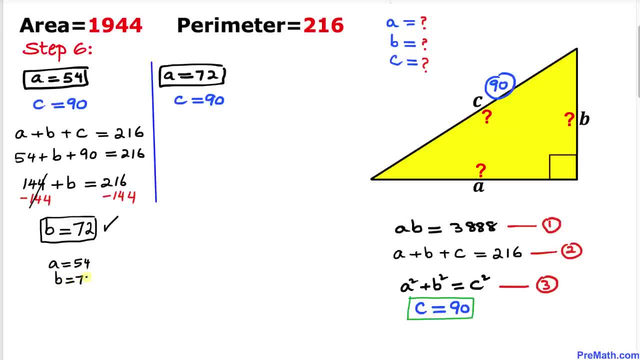 b value is 72 and c value is 90. And now let's focus on the other value of a, which is 72 c value. and now we are going to plug it in a and c value in this equation two to find the value of b. 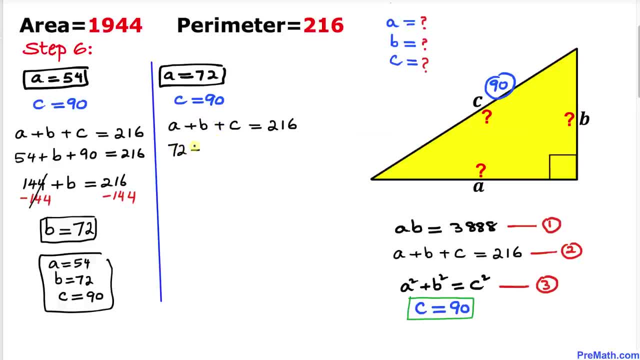 Let's go ahead and fill in the blanks: 72 plus b plus 90, equal to 216.. Now, finally, we figured out our b value as 54.. And here is ourcha result: Our a value is 72 and c value equal to 9.. So that's our b value that gave them the first of their values: dollar 22.. And now let's go ahead and fill in the blanks. So our b value is 72 plus b plus 90, equal to 216.. So finally, we figured out our b value as 54.. So thus our a value is 72 and c value is 100. And in this case our b value is 72, and then we could identify our b value as a value.